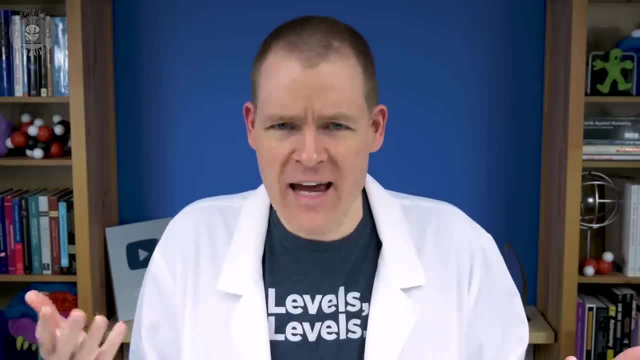 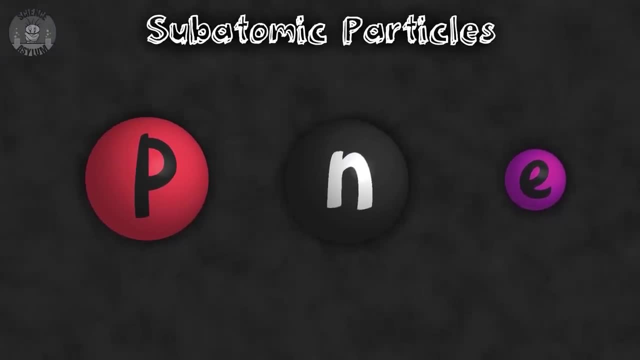 The cake is a lie. I think it's pretty common knowledge at this point that atoms are made of three things: Protons, neutrons and electrons. They're called subatomic particles for obvious reasons. Based on experiment, we know the heavy protons and neutrons are packed into a tiny nucleus. 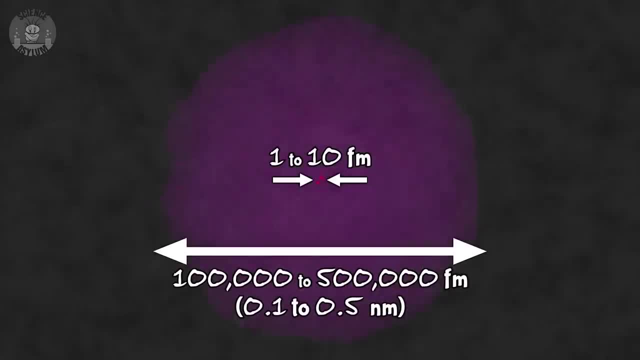 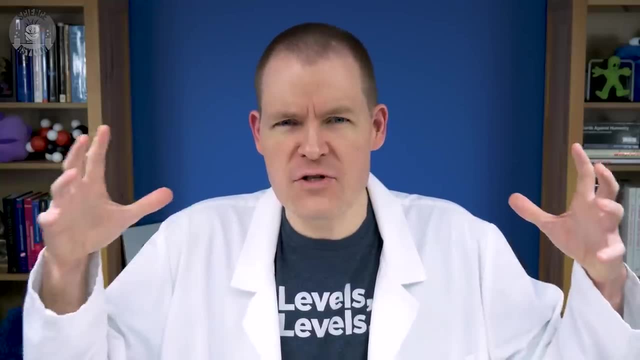 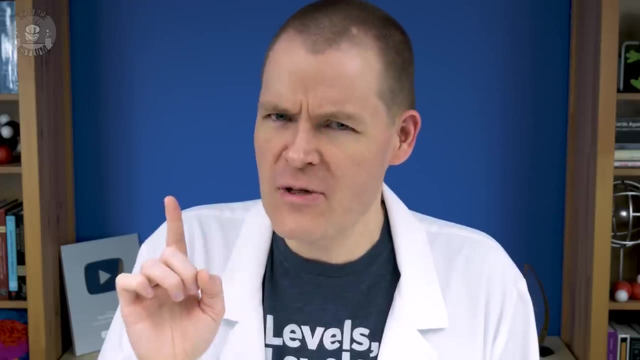 and the electrons fill a volume 100,000 times larger. The complete collection is what we call an atom. Since electrons fill the vast majority of the volume of their atom, they tend to control what their atom does. This makes understanding their behavior extremely important. 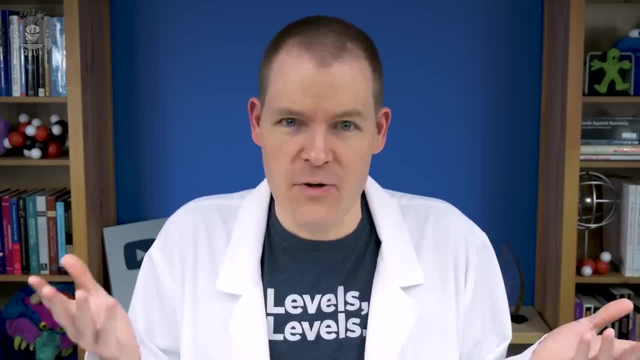 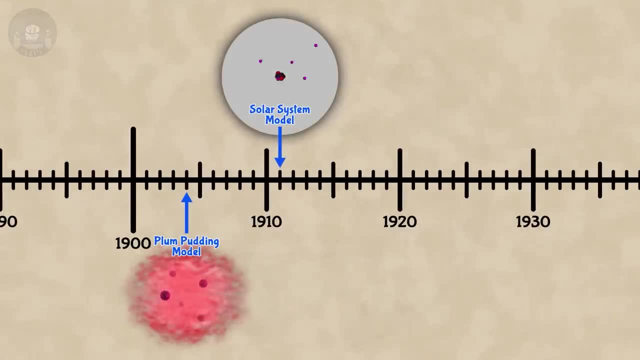 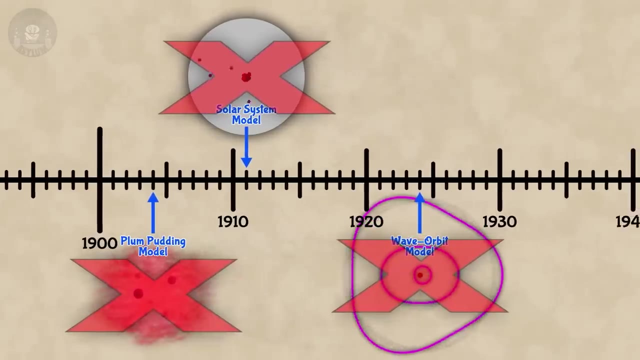 But figuring that out was a pretty difficult process. historically speaking To the timeline, We went from floating in a mist to orbits, to circular standing waves, all of which were ruled out by experiments By 1926, we were left with only one option. 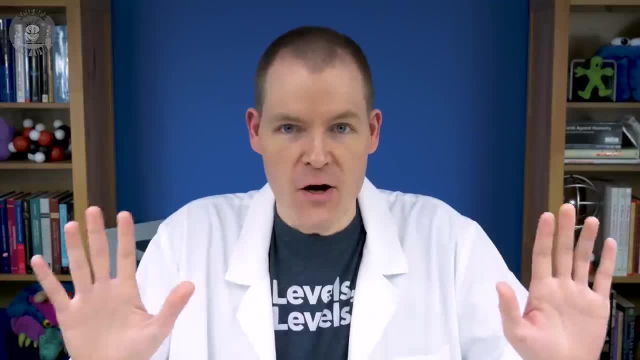 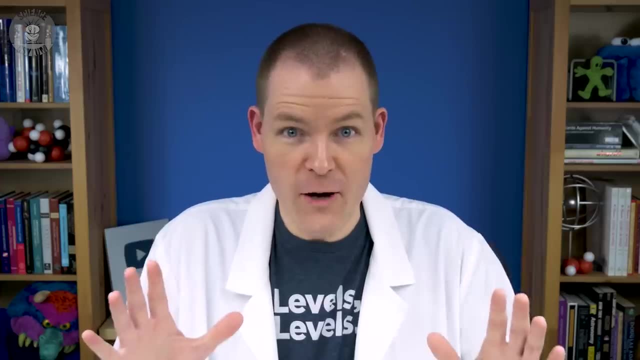 Quantum mechanics, Which, as many of you know, borders on absurdity. Quantum mechanics is weird y'all. You can quote me on that, And if we're wrong about it, the universe can only be weirder than we already think it is. 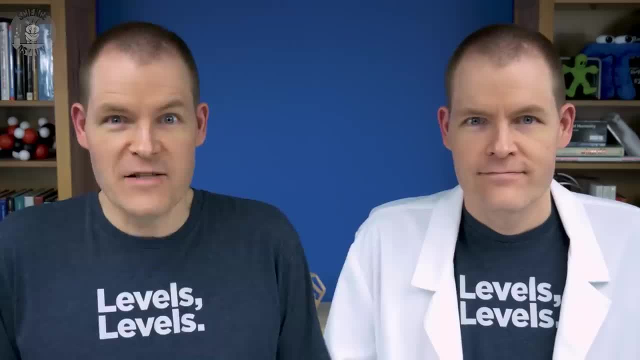 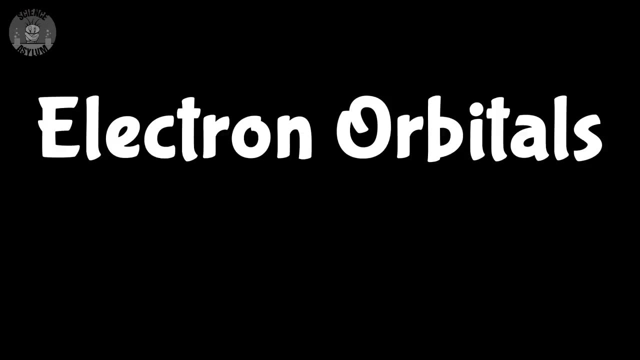 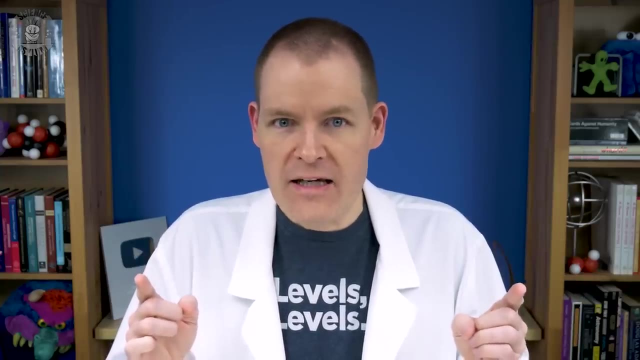 Remember we ruled out all the normal stuff. Is this where atomic orbitals come in? Yep, Let me make something absolutely clear, though: Electron orbitals are not orbits, Like at all Like any quantum state, an orbital is a state of probability. 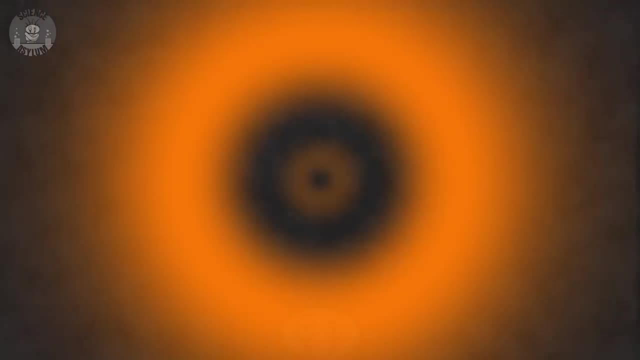 Yes, really. Here's an example of an orbital: Brighter spots are where you're more likely to find an electron, and darker spots are where you're less likely to find one. Brighter spots are where you're more likely to find an electron, and darker spots are where you're less likely to find one. 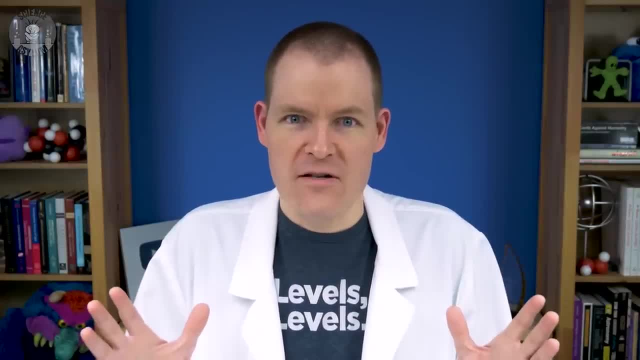 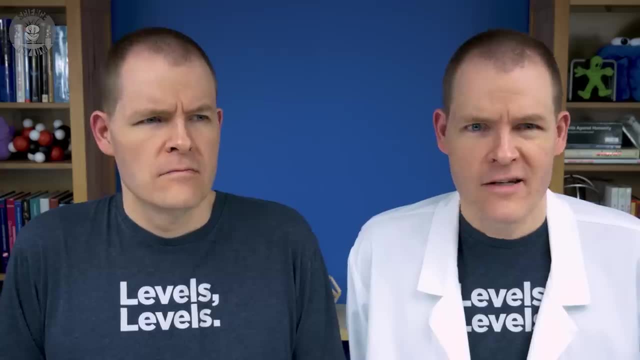 Brighter spots are where you're more likely to find an electron, and darker spots are where you're less likely to find one. The truth is, we don't actually care that much about where electrons are. Position is a pretty pointless property. What do we actually care about, then? Energy and momentum. 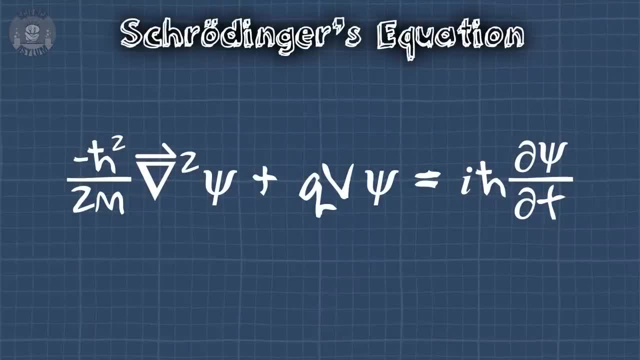 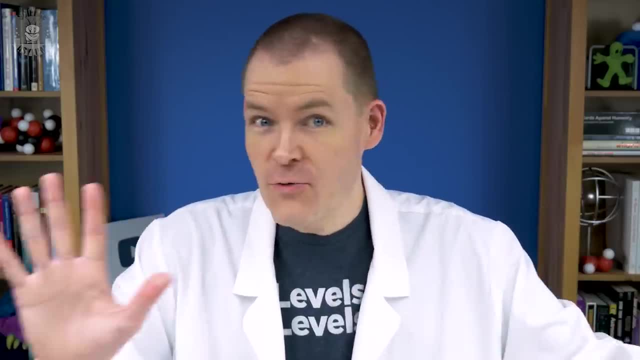 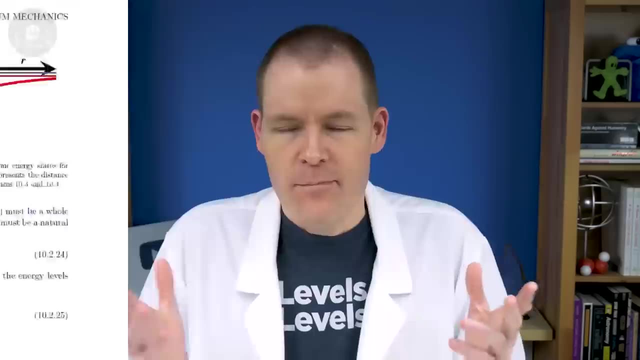 You know, conserved properties. In fact, Schrodinger's equation is an energy equation. Don't freak out, I'm not going through a full derivation or anything. If you want to see that, you'll find it in excruciating detail in my book. 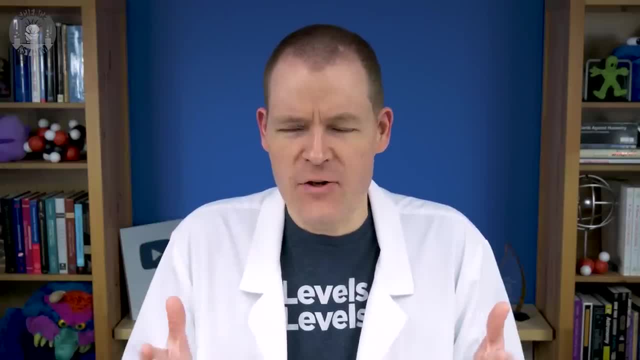 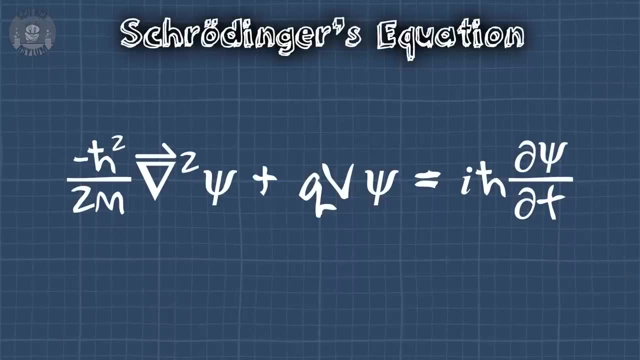 But quantum mechanics is like 90% math. If you want to learn more than just buzzwords, you're going to have to deal with at least a little math. Get on board. Anyway. this is just kinetic energy plus potential energy equals total energy. 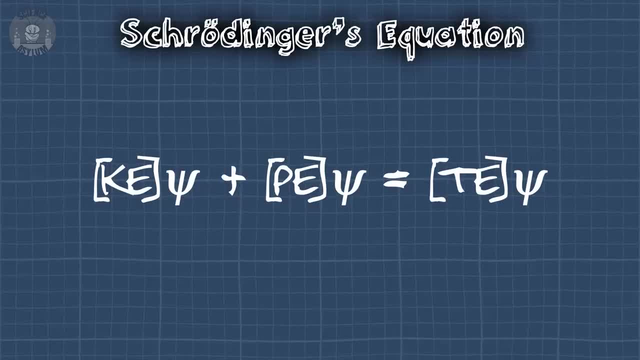 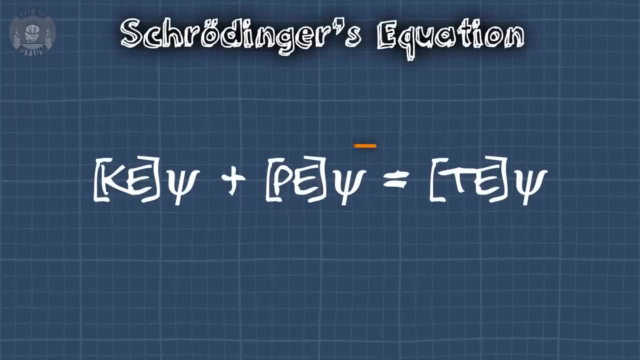 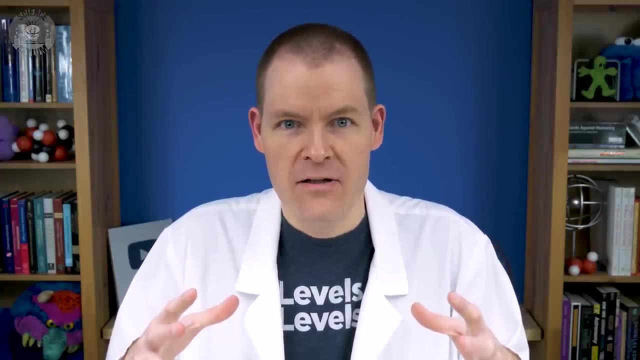 That's it. That's all. this is A quantum version of the conservation of energy. Half the battle when using this equation is figuring out what the potential energy is. In our case, it's what holds the electrons in the atom, and its influence is entirely radial. 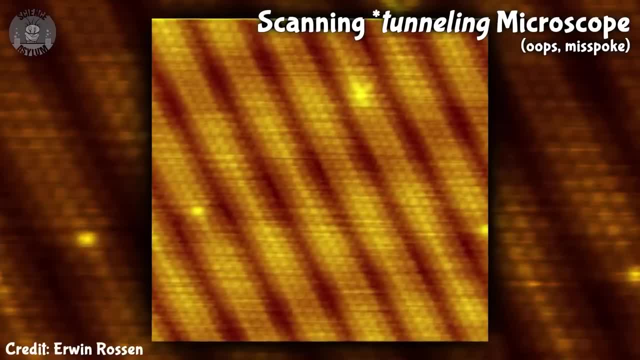 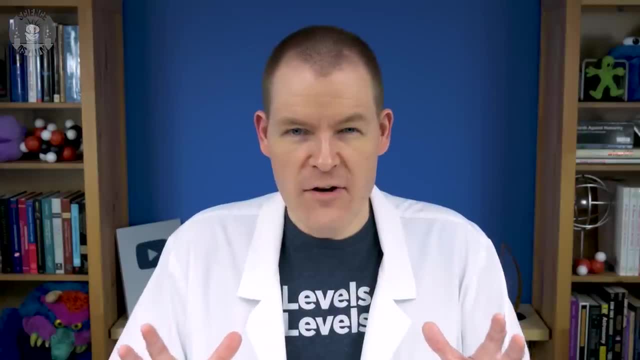 You can actually see that pretty clearly in the electron microscope image from earlier. That's why they look like tiny spheres, because their influence is radial. To take advantage of this behavior, we'll need one of my favorite tools: Spherical coordinates. They're so cool. 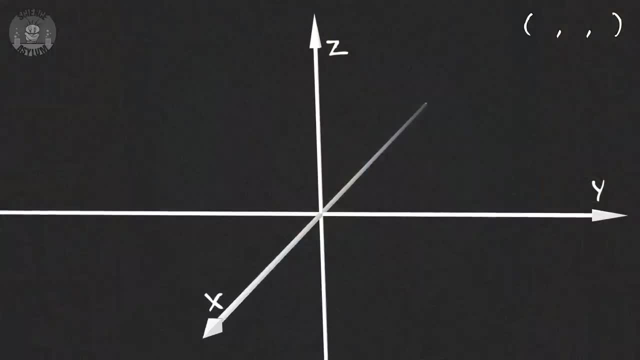 Yerrrrd Oh shush. Rather than three linear labels like X, Y and Z, we use a distance from the center, an angle from the vertical and an angle around the horizontal, Since the potential energy only depends on the distance from the center. 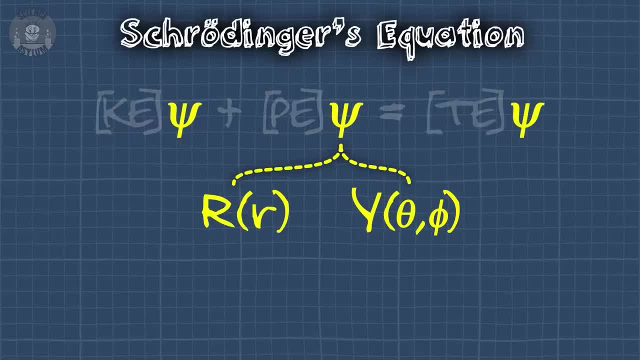 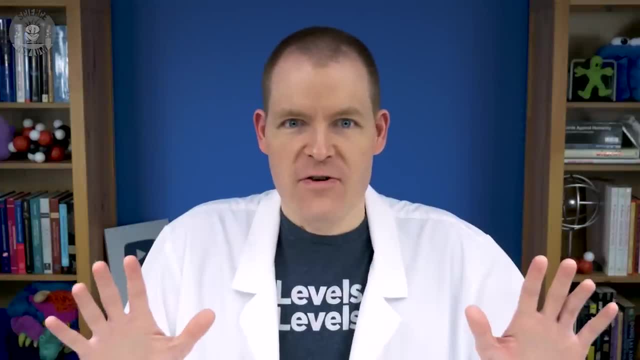 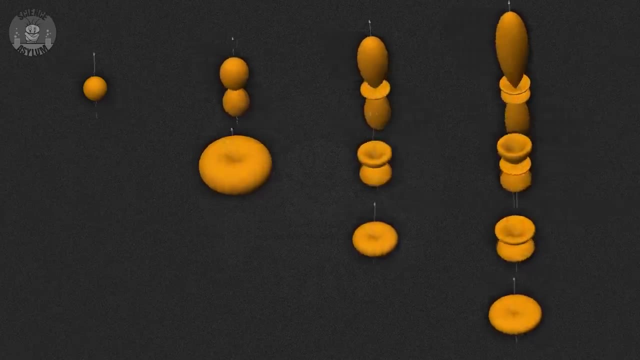 it can be separated in our solution to Schrodinger's equation. It gives us an idea of size, where the angle part gives us an idea of shape. Let's focus on the shapes first. They're called the spherical harmonics. Notice how they're all oriented along the same axis. 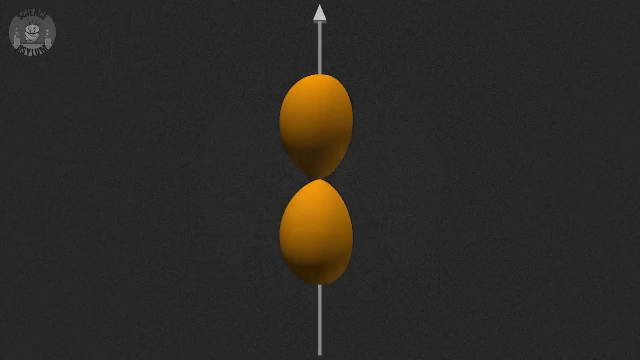 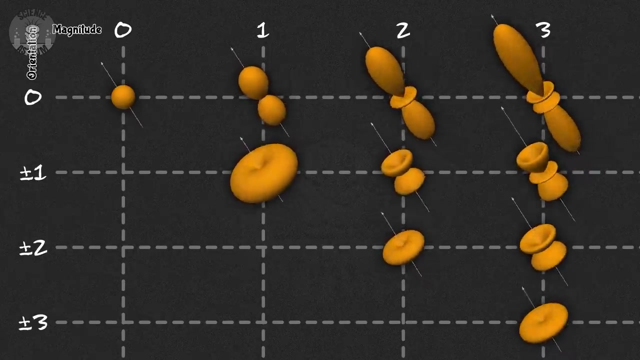 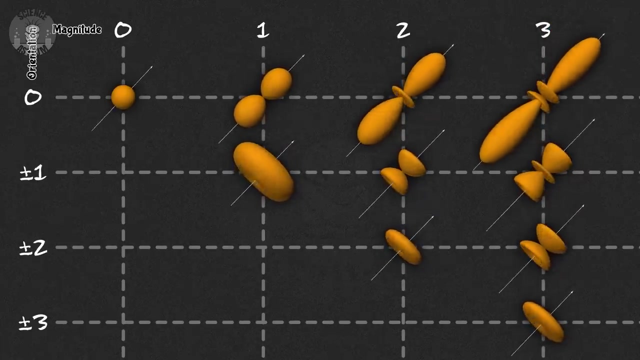 One angle draws a curve and then the other angle makes it a surface. Each one of these shapes goes with a specific angular momentum. It's what we call orbital angular momentum, because these are orbitals, not orbits. The axis they're lined up with is the direction we're measuring the momentum along. 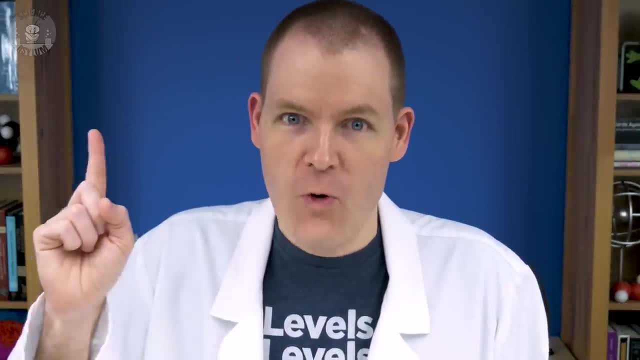 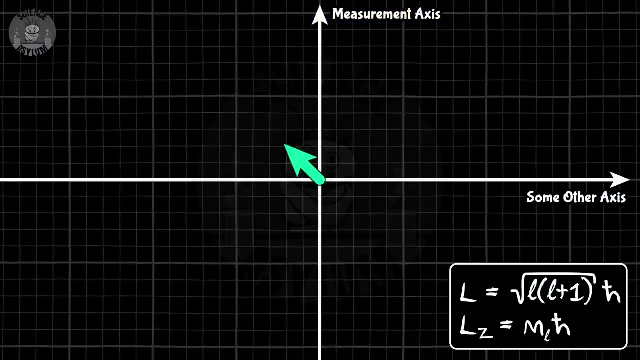 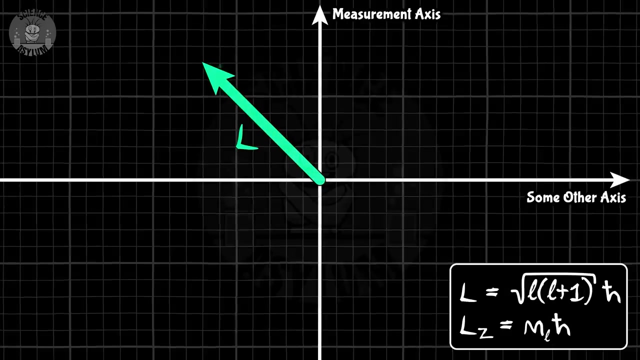 Because this is quantum mechanics. we're only allowed to measure along one axis at a time. It's kind of limited, isn't it? Yeah, but it's actually enough. One number tells us how long this angular momentum arrow is. The other number tells us its orientation. 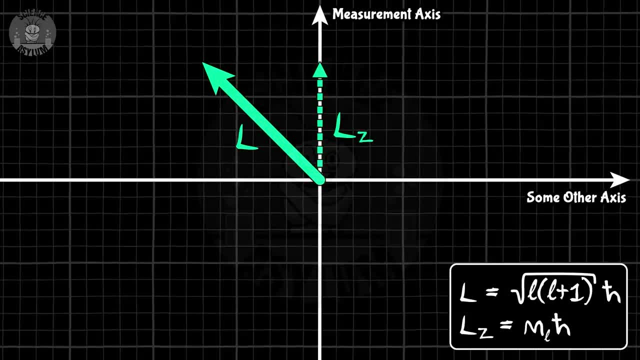 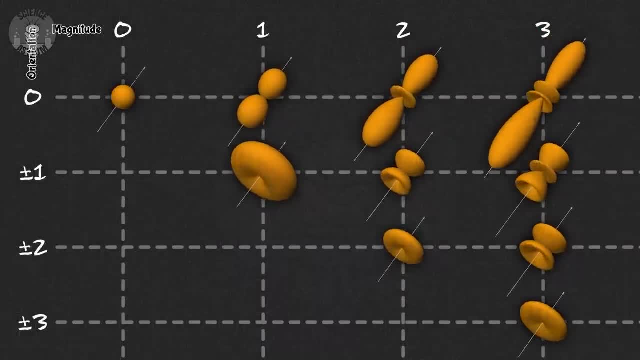 By projecting the arrow onto the measurement axis. These two numbers are all you need to know the shape of the orbital. You can even organize them into a nifty chart. like this Man, I love charts. I mean, look at this thing. 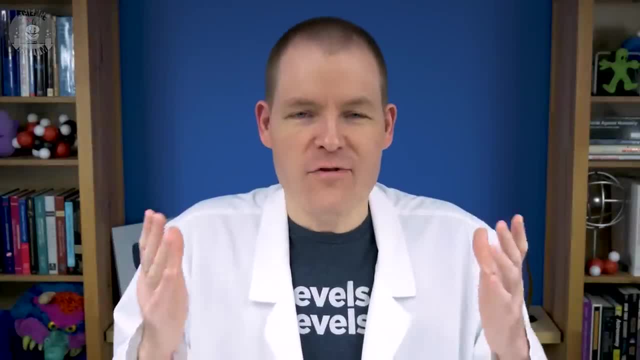 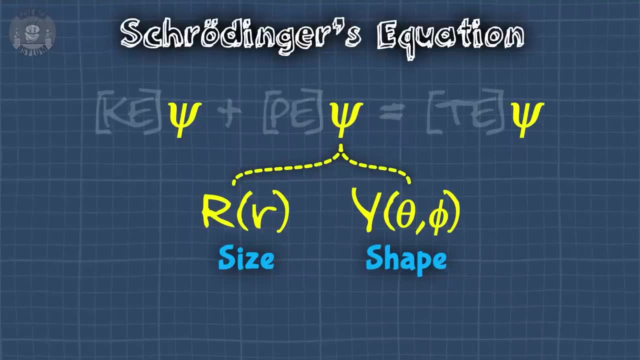 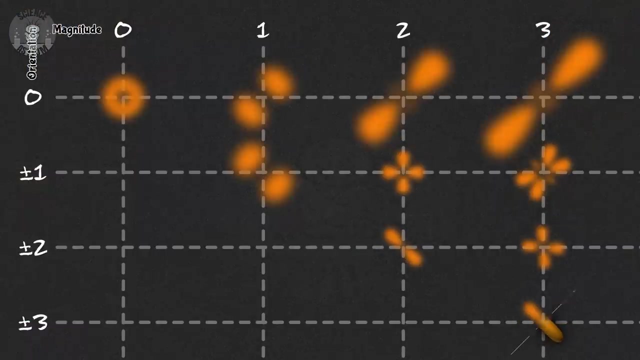 Mmm, yes, Unfortunately, none of those shapes are probability distributions yet, because we left out the radial part, It's only half. the solution. Including the radial part turns our shapes into probabilities. It turns these into these, which are further organized by energy level. 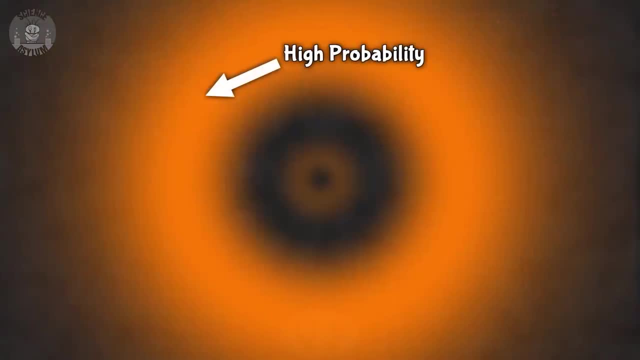 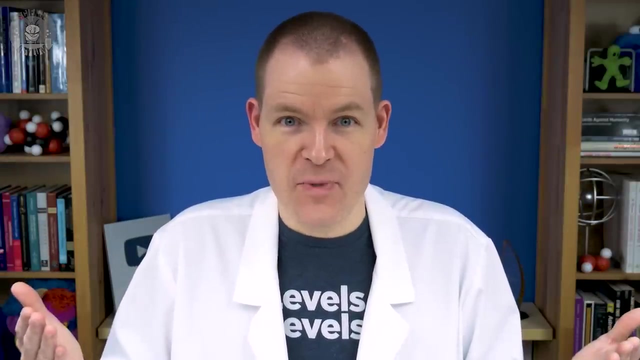 These are just probability distributions. Brighter spots are where you're more likely to find an electron. Darker spots are where you're less likely to find one. It's a visual of where you might find something if you looked. We generally don't look, though, because we want the position to be uncertain. 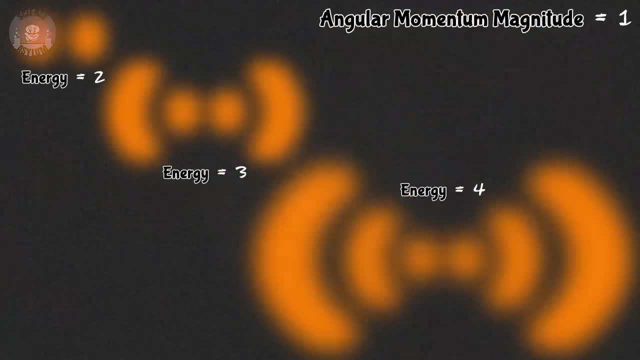 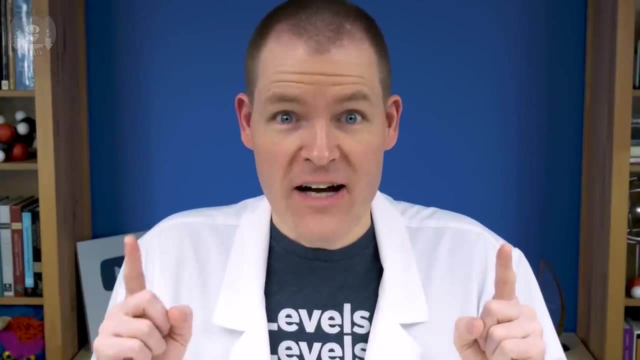 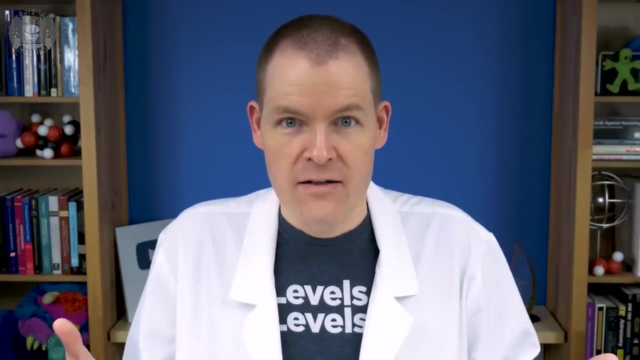 That way the energy and angular momentum remain definite for each state. But like I said at the beginning of the video, this all looks pretty static. Atomic orbitals are actually dynamic. An electron can absorb and release photons which can change that electron's energy. 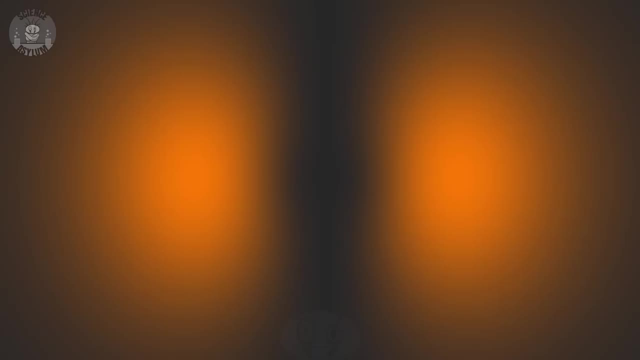 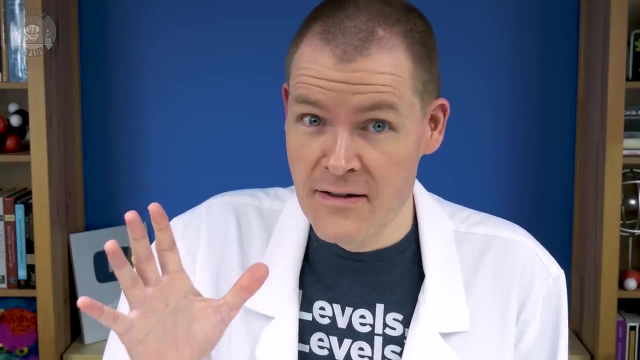 Electrons can jump between quantum states. Based on what I've mentioned so far, you're probably only imagining a simple fade, But it's actually way cooler than that. Quantum mechanics might be weird, but it's still a set of rules. The events might be probabilistic. 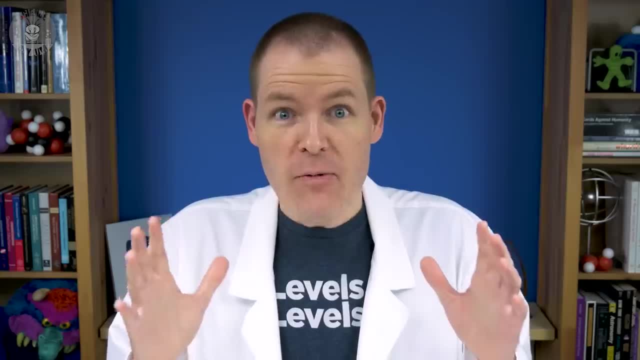 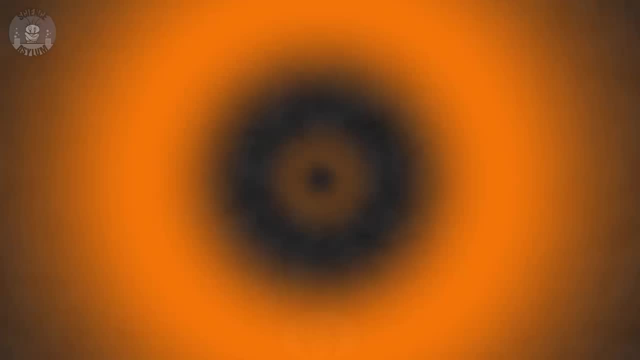 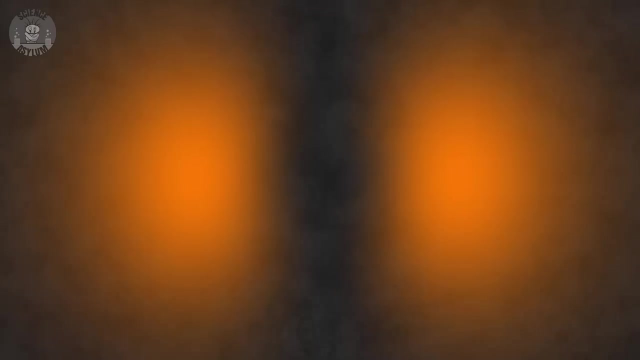 But the probabilities are deterministic And that probability must be conserved, just like energy and momentum. That means you can imagine probability as if it's a fluid filling all of space. When the distribution changes, that probability has to flow to the new locations. 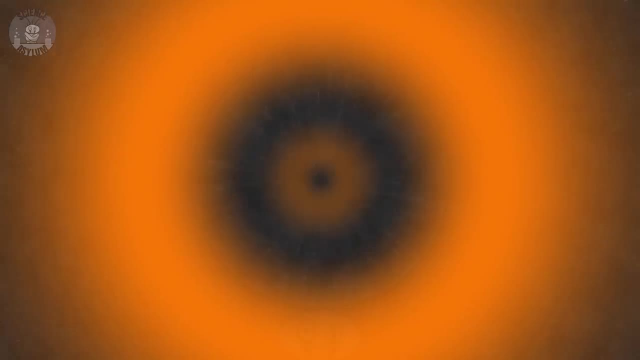 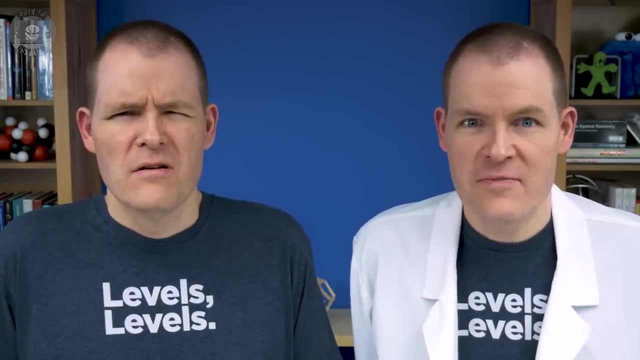 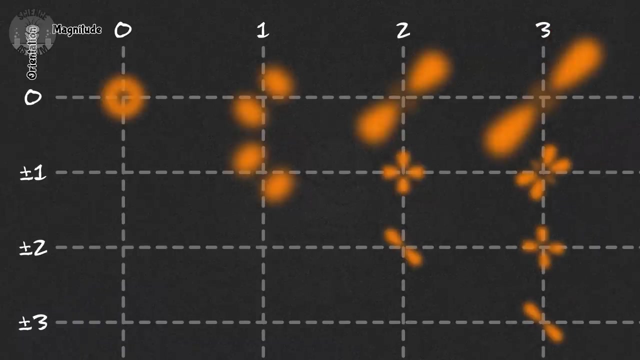 Orbital transitions look more like this: That flow is called a probability current, Kind of cool huh. So what's an atomic orbital? A quantum state of probability. The angular momentum tells us the shape, The energy fills the volume of that shape with detail and gives us an idea of size. 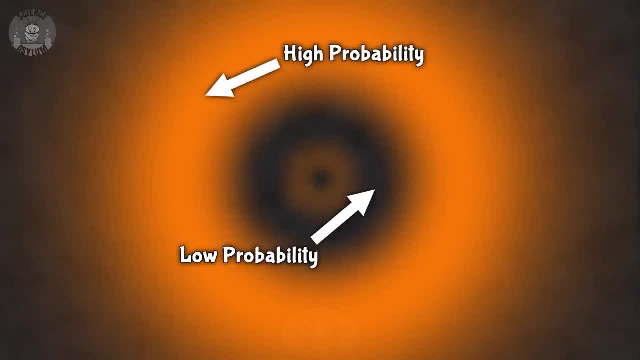 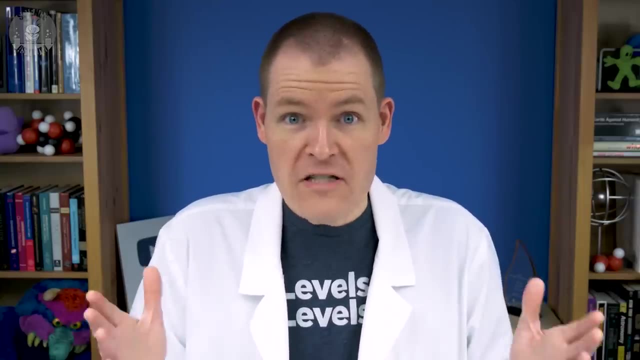 Brighter spots are where you're more likely to find an electron. Darker spots are where you're less likely to find one. But the probability of finding the electron somewhere must be 100% at all times. Quantum probability must be conserved.